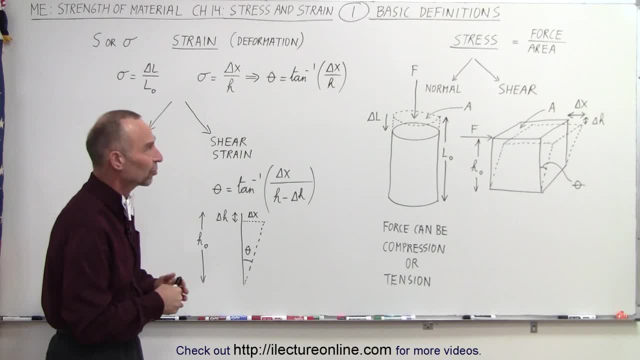 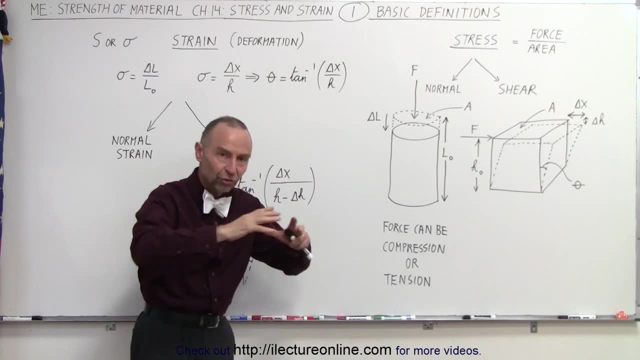 we'll talk about some basic definitions regarding stress and strain. When we're stressing a material, we're applying a force, And usually that material has a certain cross-sectional area. So the stress is then defined by the ratio of the amount of force applied divided by the 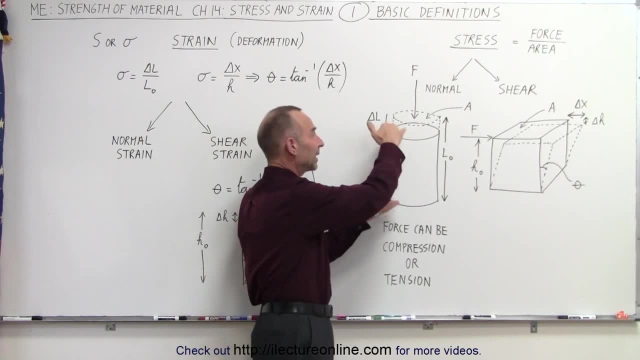 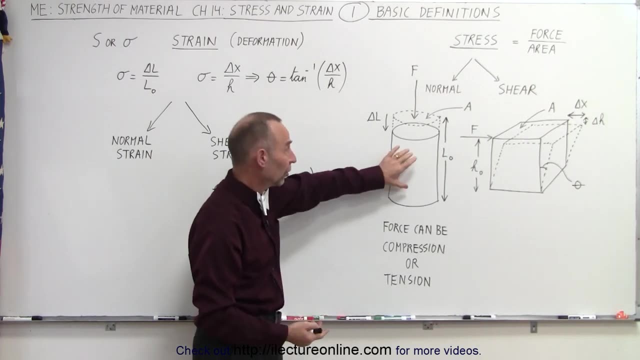 cross-sectional area of the material. This could be a beam, this could be a cable, this could be a bar or anything like that, And so the force can either be a compression force if this is a solid material such as a bar or a beam or something like that. 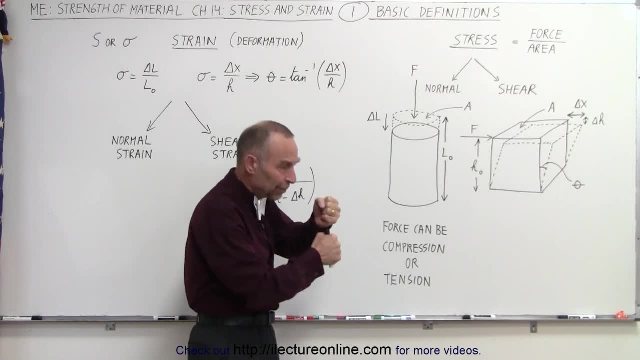 or it can be a tension force. In other words, if it's a cable, then of course you can't really compress the cable in that direction You want to pull on the cable, then we have what we call a tension force. If we then divide that force by the cross-sectional area of the object, 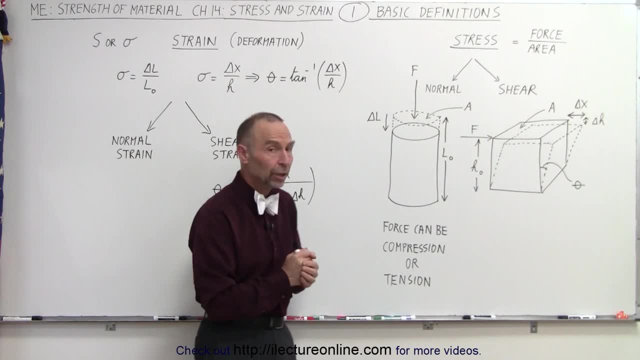 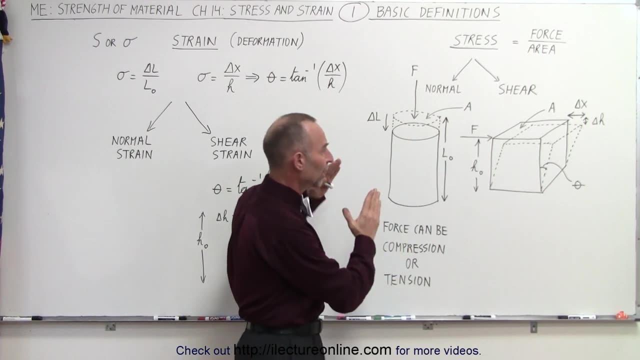 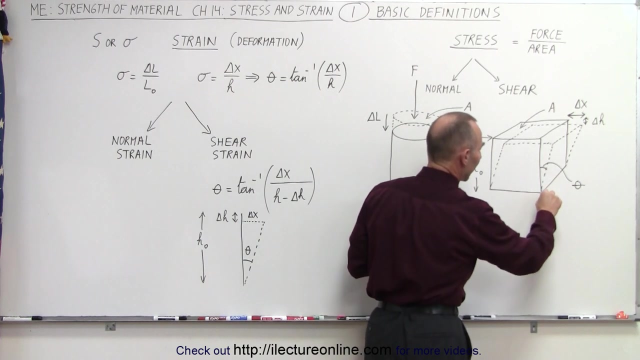 then we have what we call the stress on the material. We can also have a shear stress, which is where the force is applied laterally to the material so that we push it out of its normal shape. You can see if this is a block here, and of course we probably want to have something over here. 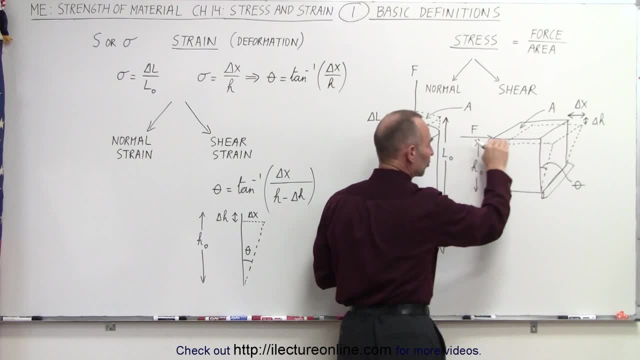 to keep the block from sliding. And then if we push on the top end of the block, you see, we'll deform the block that way. Notice that the block will be pushed to the right so that the top portion will move a delta x to the right. 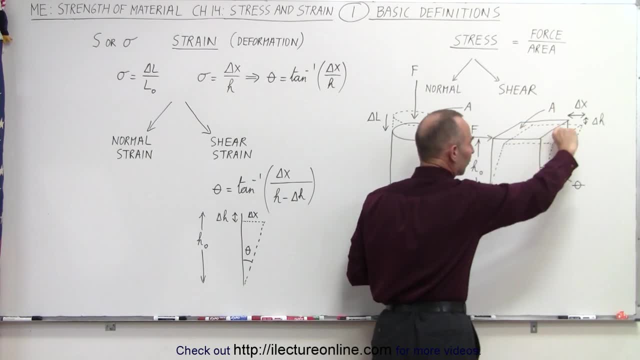 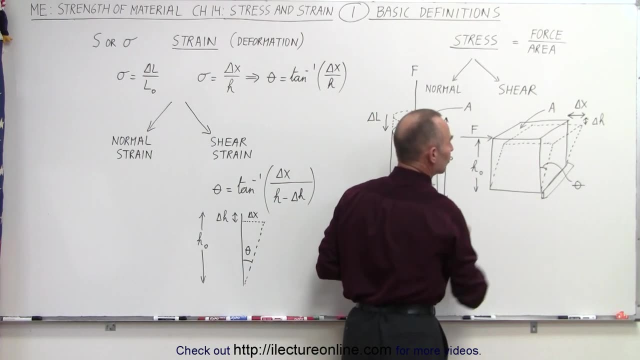 And sometimes also depending upon the shape, if it's pushed far enough, we can also take into account the difference in the height of that block, and then we'll form an angle of deformation here. So we either have what we call a normal stress, where the force is normal to the cross-sectional area. 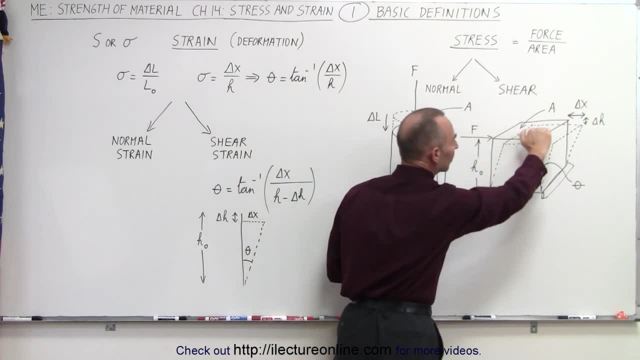 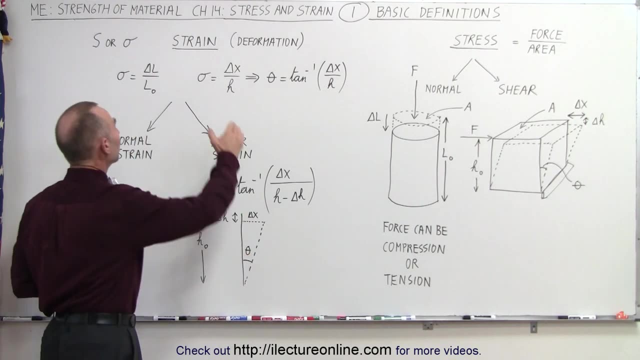 or we have a shear stress, where the force is parallel to the cross-sectional area- another way of looking at it: When we apply a stress to material, we usually end up with what we call a strain to the material. A strain is defined as the deformation, a change in the shape. 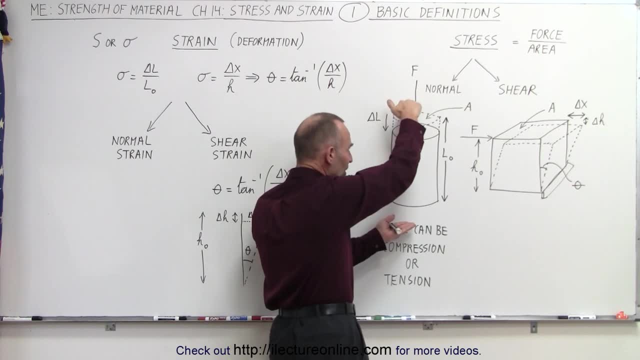 Notice, when we have a bar or beam and we push down on it, we'll change the length of that beam. We'll change the length by a small amount and that's called the deformation. Actually, the change in length divided by the original length is actually the way the deformation, or the strain, is defined. 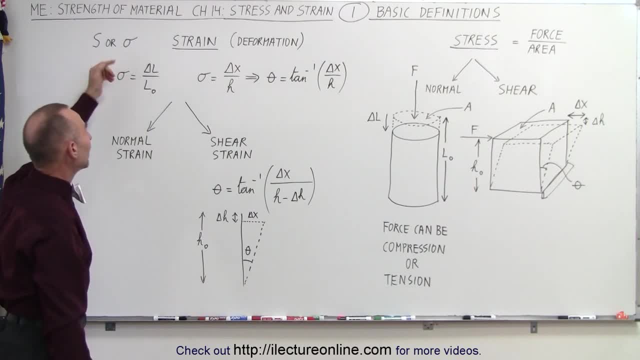 Notice we can use the letter s or the letter sigma to indicate strain, because both start with s, as the s sound, So sigma. the strain is defined as the change in the length divided by the original length when we're talking about the normal stress. 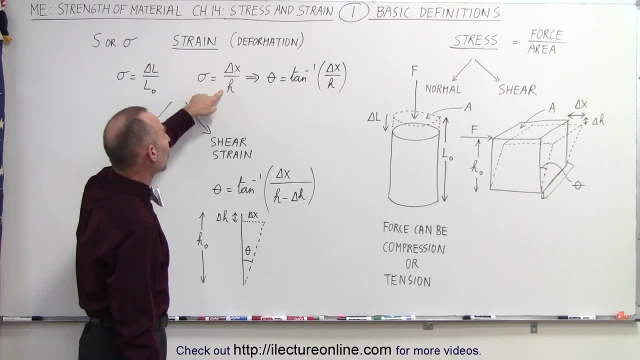 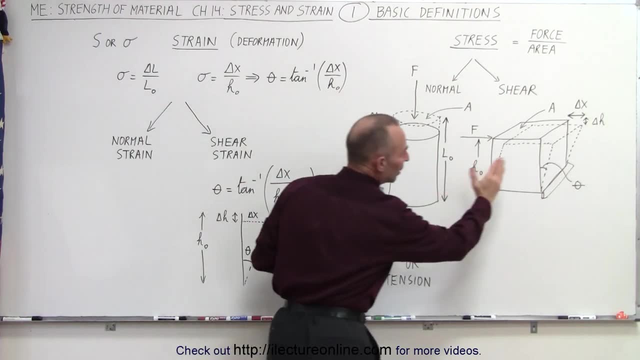 And the strain can also be defined as the change in x over the original length. We probably want to put the original height down like this, such that the angle of deformation, as you can see here in the drawing, can be defined as the inverse tangent of that ratio. 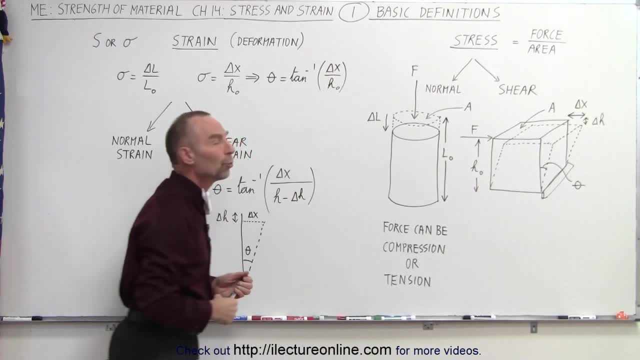 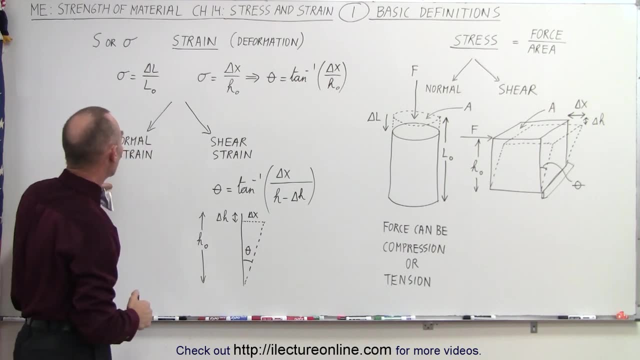 the change in the horizontal displacement divided by the original height of the object that we're shearing, that we're applying a shear stress to it. So we have what we call the normal strain, where the strain is in the direction of the force. 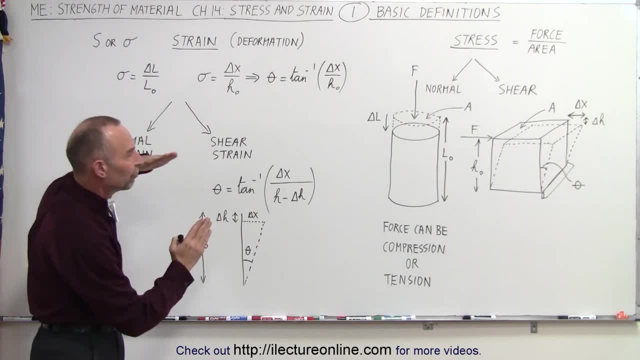 or we can talk about the shear strain, where we deform the force, The object, where we can see that the force applied perpendicular to the area of the object. Sometimes we need to take into account that there's a slight change in the height, a small delta h, and so then the angle of strain, the strain angle. 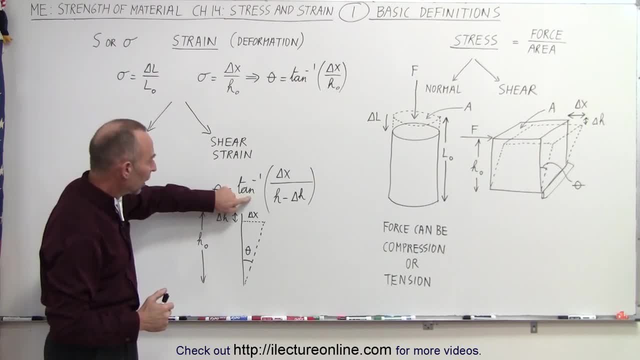 can then be defined as the inverse tangent of delta x divided by h minus the delta h. I'll go ahead and call it h sub naught, And so then, sometimes we do have to take that into account, because that'll make a small amount of difference. 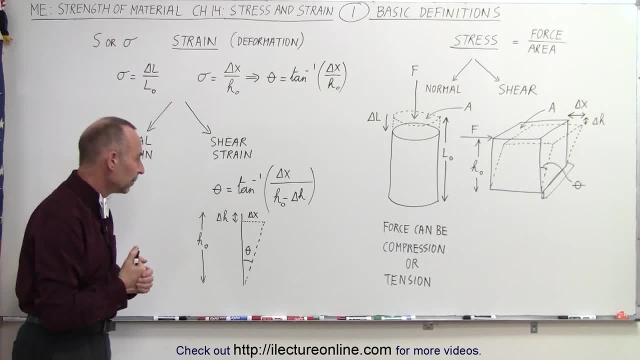 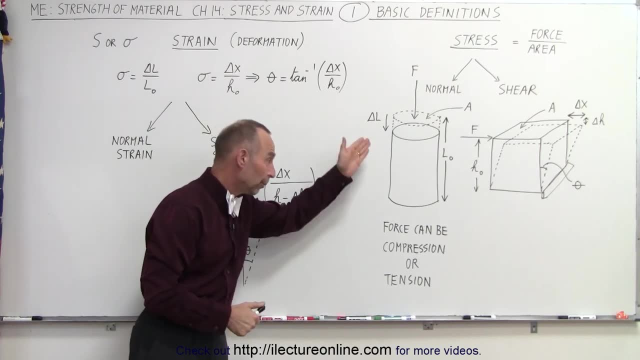 If delta h is very small, we can just go ahead and ignore it. Now notice again that the force can be a compression or a tension force when it's in the perpendicular or normal direction. Typically when we talk about cables, it'll be a tension force. 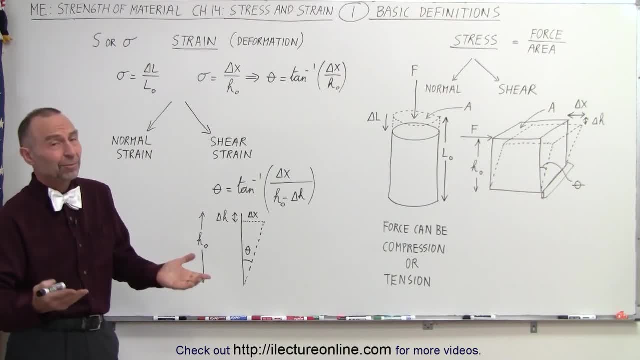 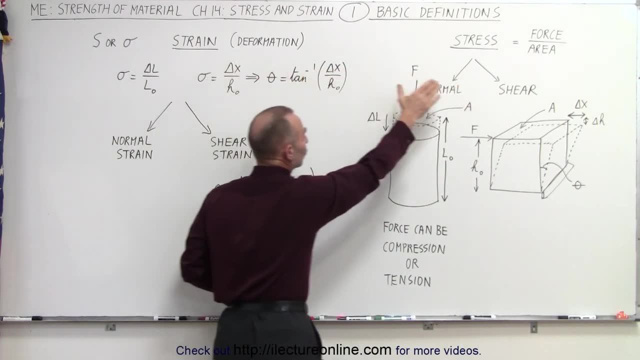 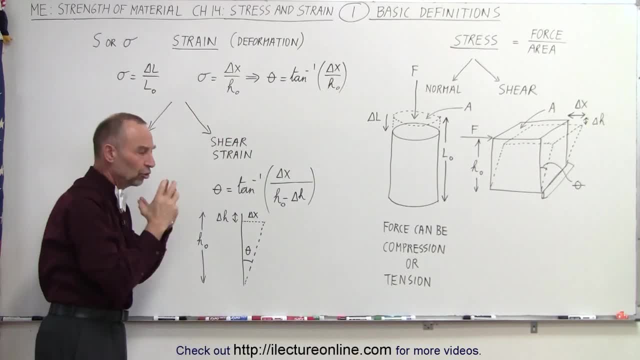